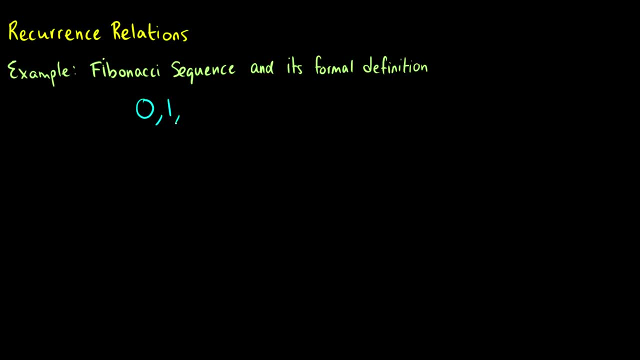 So we start off with the numbers 0 and 1, and then the next number in the sequence is always going to be the previous two added together. So 0 plus 1 is 1,, 1 plus 1 is 2,, 1 plus 2 is 3,. 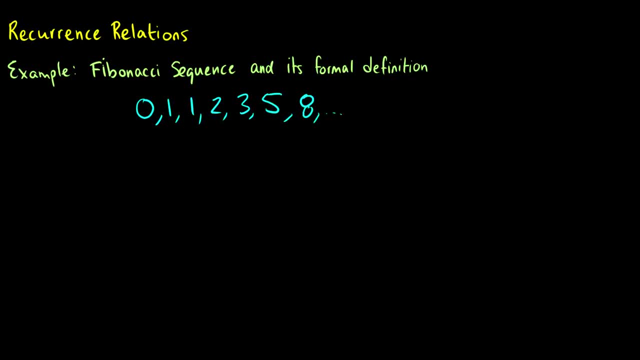 2 plus 3 is 5,, 3 plus 5 is 8, so on and so forth. So that's the counting sequence. More formally, we can define the nth number, a n, to be equal to the sum of the two previous numbers. 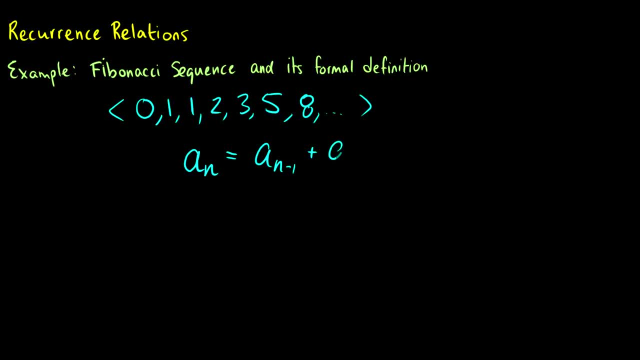 So we can say this is a n minus 1 plus a n minus 2.. Commonly you'll see this with Fibonacci written f n is equal to f n minus 1 plus f n minus 2.. I'm just going to use a's to be consistent with all of my examples. 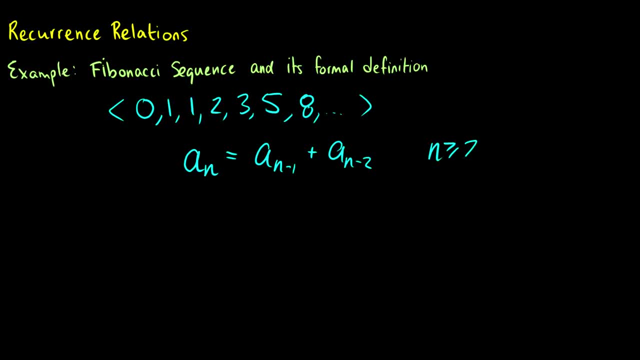 So this is for n greater or equal to 2, because we don't want a of negative 2, because we can't have the negative 2th number in a sequence doesn't make any sense. So we have a n is equal to a n minus 1, plus a n minus 2,. 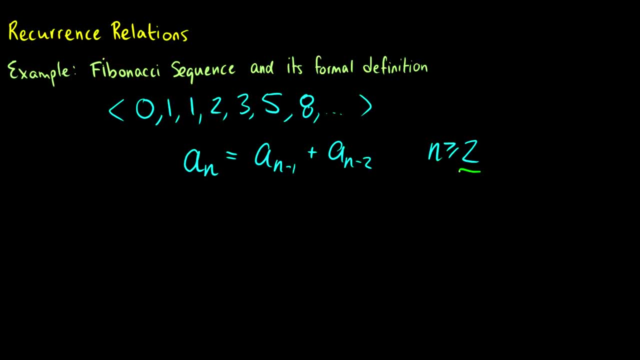 the problem is right now is that n has to be greater than or equal to 2.. So a 2 is equal to a 1 plus a 0, but I haven't defined what a 1 and a 0 are yet. We need those two, so we'll start off the sequence by saying that a 0 is equal to 0. 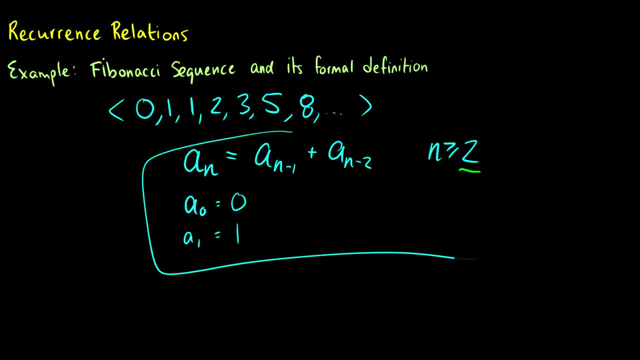 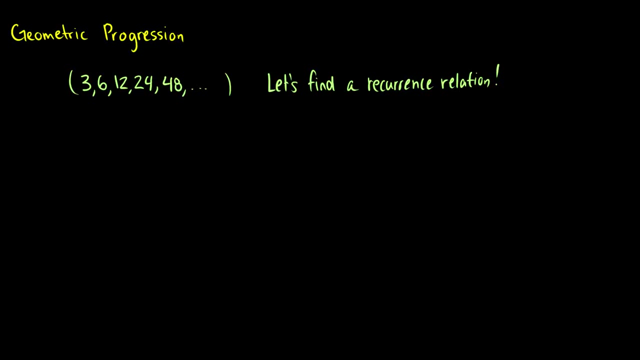 and a 1 is equal to 1, and that is the formal definition of the Fibonacci sequence. So let's take a look at another type of sequence, a geometric progression. Okay, so 3,, 6,, 12,, 24,, 48. Okay, this seems pretty straightforward. 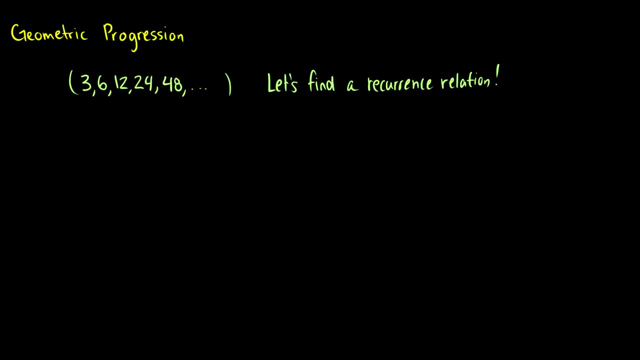 Let's write out a formal definition for this. Okay, a n is equal to okay. if we take some nth number, some arbitrary number, in fact, let's take 48. How do we get 48?? Well, we take the previous number, a n minus 1, and then we multiply by 2.. 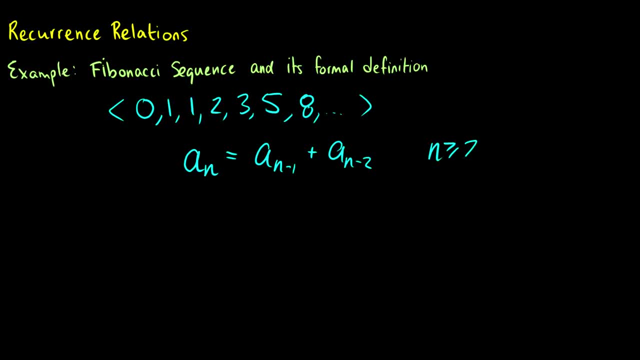 So this is for n greater or equal to 2, because we don't want a of negative 2, because we can't have the negative 2th number in a sequence doesn't make any sense. So we have a n is equal to a n minus 1, plus a n minus 2,. 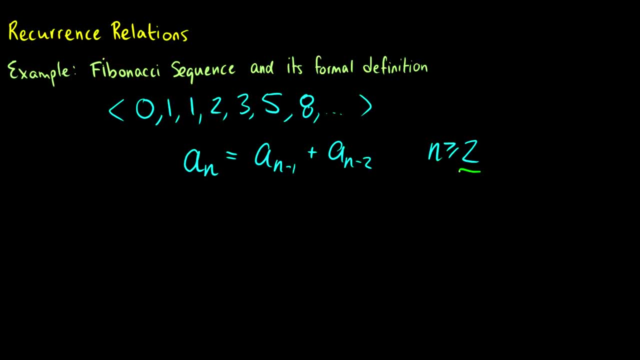 the problem is right now is that n has to be greater than or equal to 2.. So a 2 is equal to a 1 plus a 0, but I haven't defined what a 1 and a 0 are yet. We need those two, so we'll start off the sequence by saying that a 0 is equal to 0. 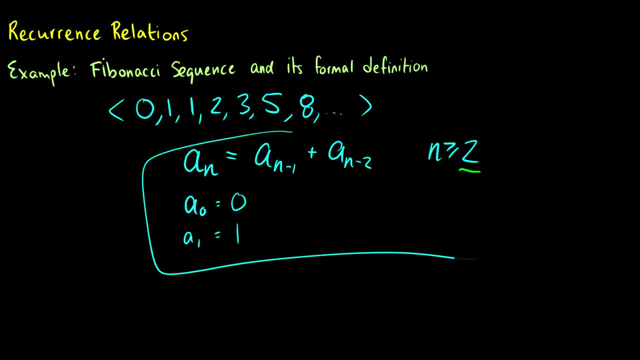 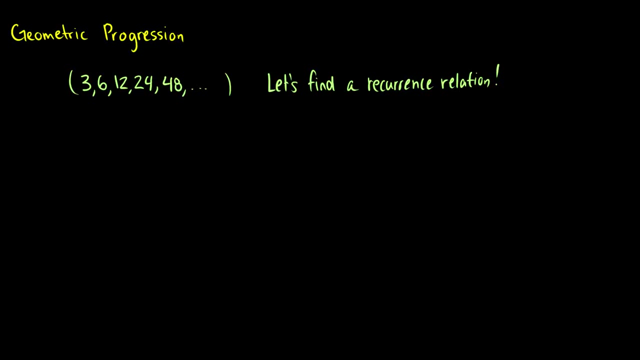 and a 1 is equal to 1, and that is the formal definition of the Fibonacci sequence. So let's take a look at another type of sequence, a geometric progression. Okay, so 3,, 6,, 12,, 24,, 48. Okay, this seems pretty straightforward. 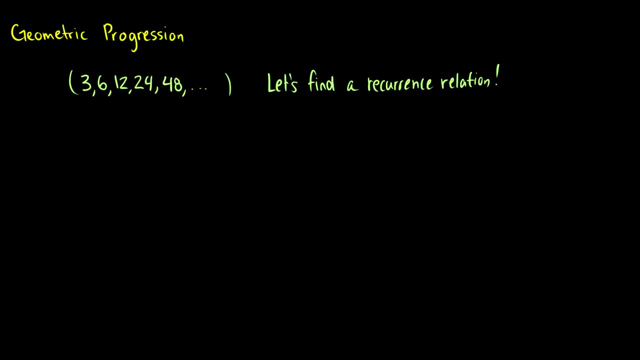 Let's write out a formal definition for this. Okay, a n is equal to okay. if we take some nth number, some arbitrary number, in fact, let's take 48. How do we get 48?? Well, we take the previous number, a n minus 1, and then we multiply by 2.. 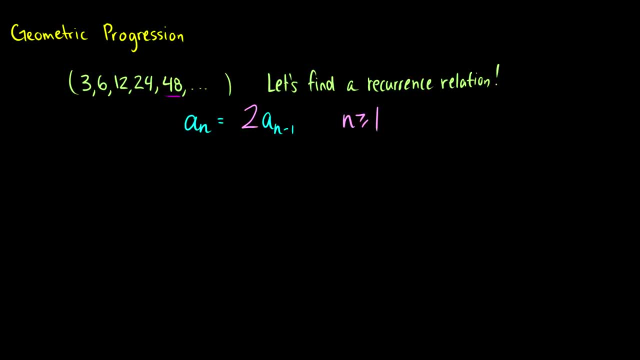 And of course, this has to be for n greater or equal to 1, because we need one previous number to figure out what the current number is. And what is the first number in the sequence to start it off? Well, that's the number 3.. So this is the recurrence relation for this sequence. 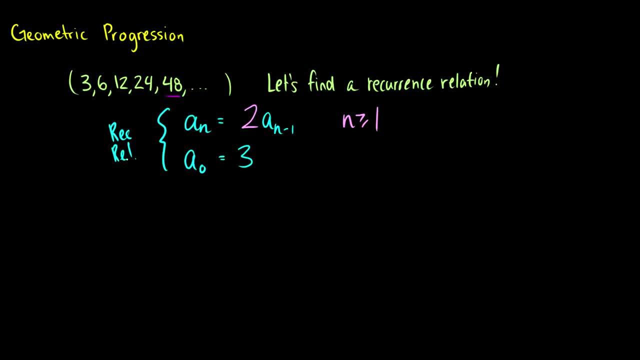 Now, what's nice about this is that we can figure out a5,, a8,, a12, and figure out whatever we want. The only problem is when I say, hey, what's a of 667?? Well, that's going to be 2 times a of 666,, but hold on a second. what's a of 666?? 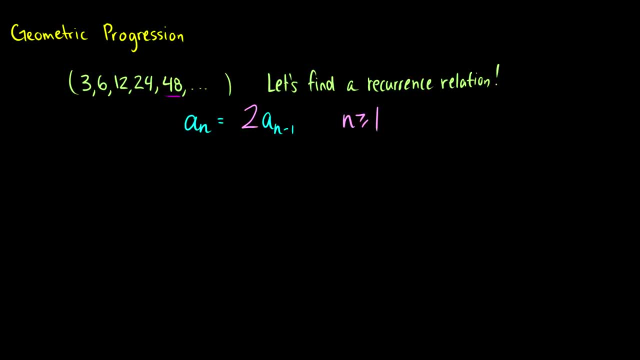 And of course, this has to be for n greater equal to 1, because we need one previous number to figure out what the current number is. And what is the first number in the sequence to start it off? Well, that's the number 3.. So this is the recurrence relation for this sequence. 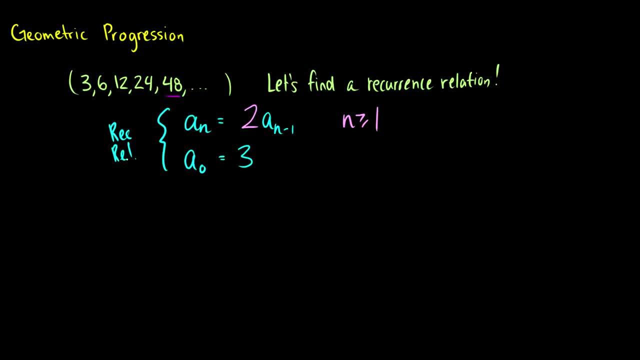 Now, what's nice about this is that we can figure out a5,, a8,, a12, and figure out whatever we want. The only problem is when I say, hey, what's a of 667?? Well, that's going to be 2 times a of 666,, but hold on a second. what's a of 666?? 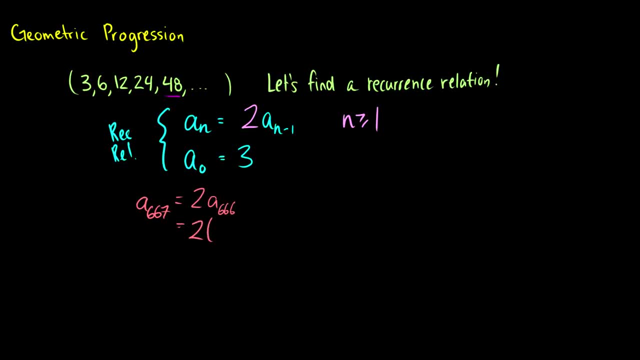 Well, we just need to figure out that a of 666 is just 2 times a of 665.. Okay, so if you know a of 665, then you can figure out a666 and a667,, but that's kind of an absurd claim because that's a lot of unnecessary computation. 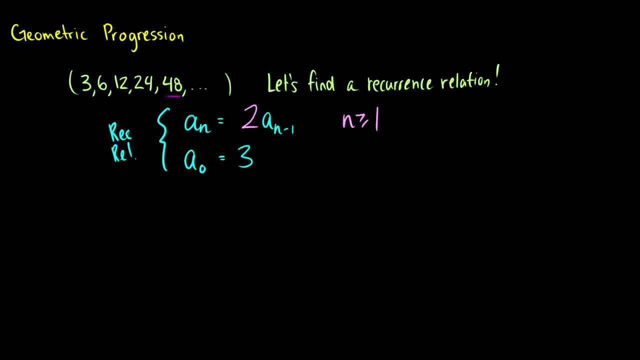 What we want is a way to solve this for a formula. So let's solve a. n is e, Okay. well, the first number we want is 3, so we want a of 0 to equal 3.. So what's a good way of doing that? 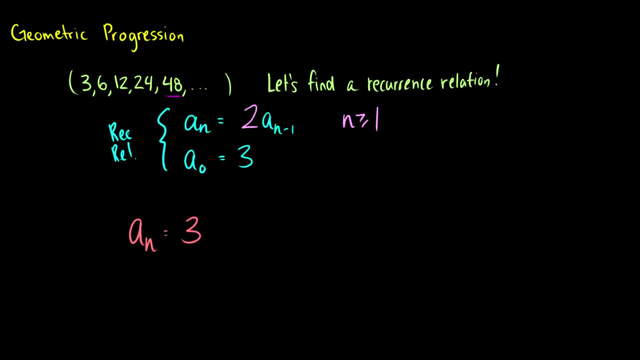 Well, we could take our number 3, and okay, we have 3,, but this needs to be multiplied by something. So a1 is going to be 6,, a2 is going to be 12, so why don't we multiply it by 2 to the? 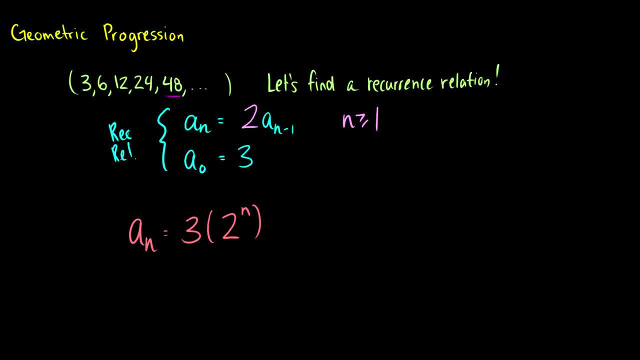 n. Okay, So a0 is just 3 times 2 to the 0 is 1.. Okay, that's good. a to the 1 is equal to 3 times 2 to the 1.. 3 times 2 is 6.. 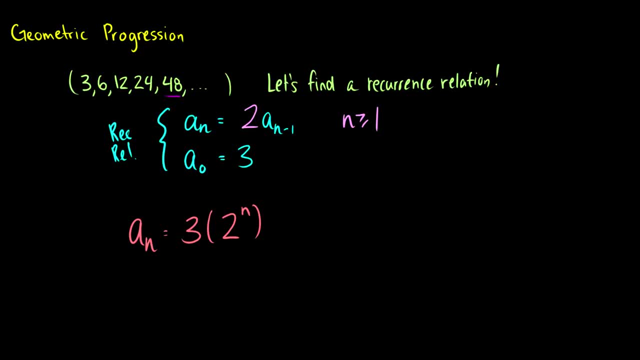 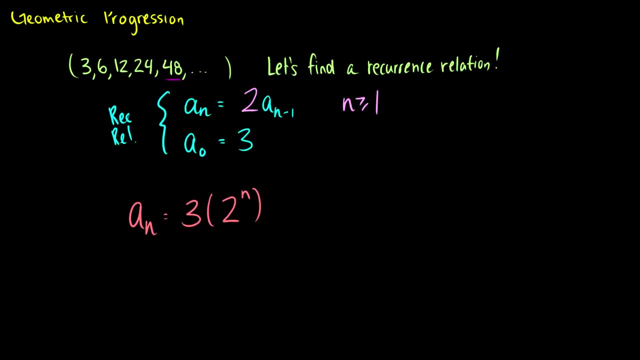 Okay, that looks good. a of 2 is 3 times 2 to the 2, so 3 times 4 is equal to 12.. Okay, that seems pretty good. So here's how geometric progression solutions work, and these are unique because these: 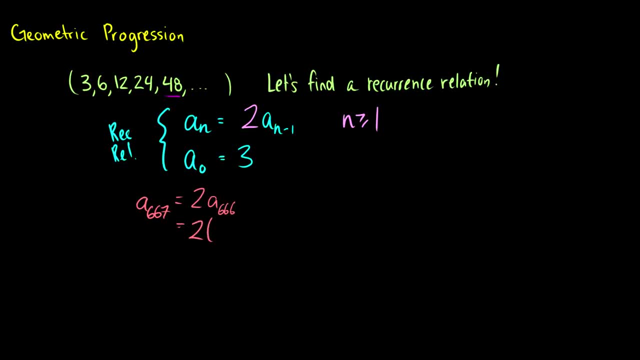 Well, we just need to figure out that a of 666 is just 2 times a of 665.. Okay, so if you know a of 665, then you can figure out a666 and a667,, but that's kind of an absurd claim because that's a lot of unnecessary computation. 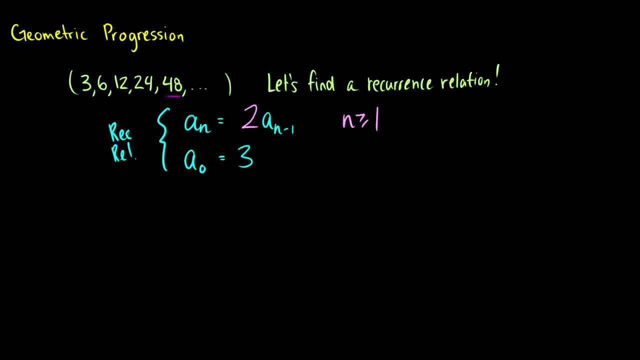 What we want is a way to solve this for a formula. So let's solve a. n is e, Okay. well, the first number we want is 3, so we want a of 0 to equal 3.. So what's a good way of doing that? 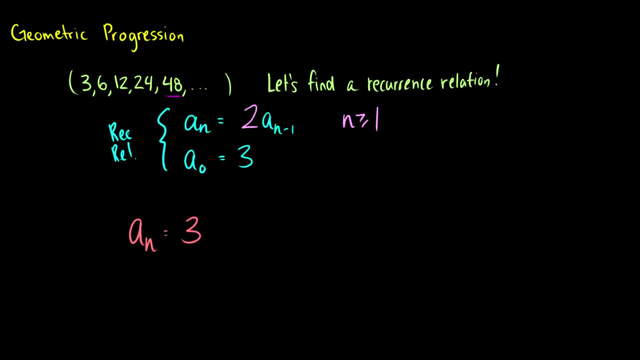 Well, we could take our number 3, and okay, we have 3,, but this needs to be multiplied by something. So a1 is going to be 6,, a2 is going to be 12, so why don't we multiply it by 2 to the? 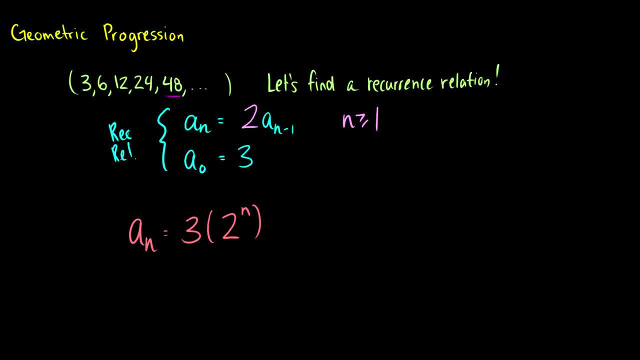 n. Okay, So a0 is just 3 times 2 to the 0 is 1.. Okay, that's good. a to the 1 is equal to 3 times 2 to the 1.. 3 times 2 is 6.. 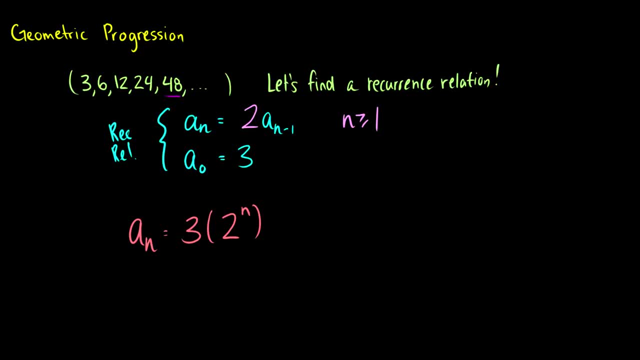 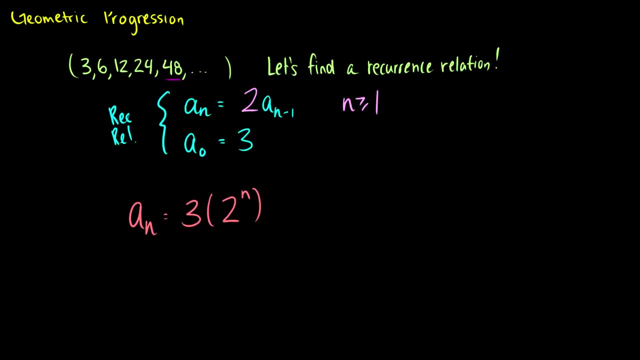 Okay, that looks good. a of 2 is 3 times 2 to the 2, so 3 times 4 is equal to 12.. Okay, that seems pretty good. So here's how geometric progression solutions work, and these are unique because these: 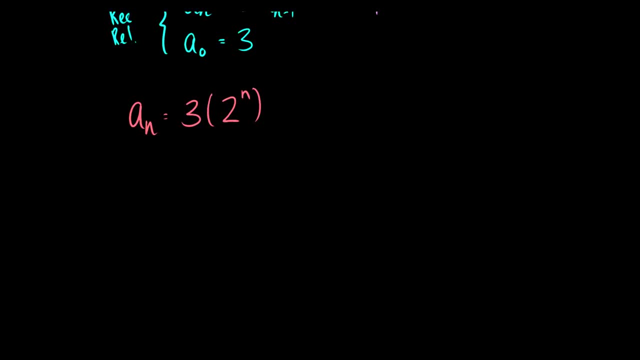 are fairly straightforward ways to solve these relationships. These are very nice. If we have a relation, an is equal to d times an minus 1, so d is just our constant and a0 is equal to some number, k, then we can summarize this formula as an is equal to k. 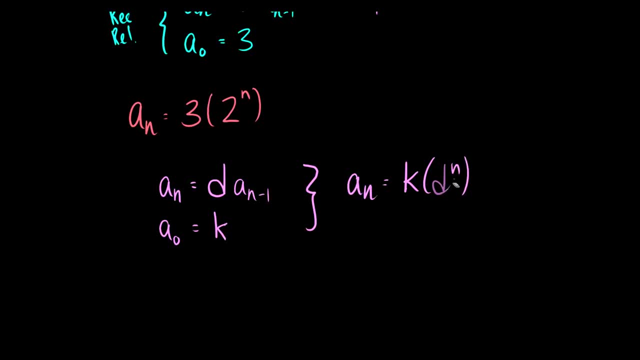 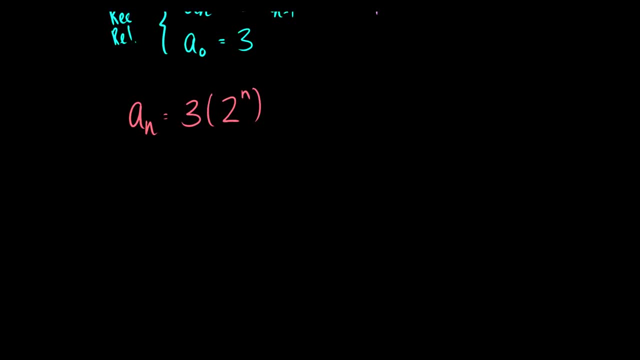 are fairly straightforward ways to solve these relationships. These are very nice. If we have a relation, an is equal to d times an minus 1, so d is just our constant and a0 is equal to some number, k, then we can summarize this formula as an is equal to k. 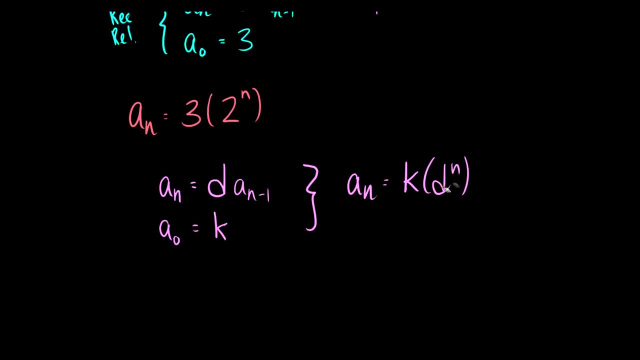 times d to the n. Okay, And of course this is going to be for n greater or equal to 0.. This section is going to be n greater or equal to 0.. And this recurrence relation is going to be n greater or equal to 1.. 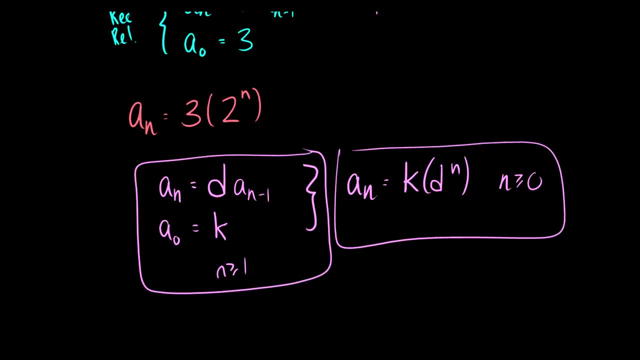 So these are two different ways of looking at things. One is a recurrence relation, The other is a nice formula that allows us to compute any number without needing to know the previous numbers. So that's great, But what can happen is we can get some more tricky examples. 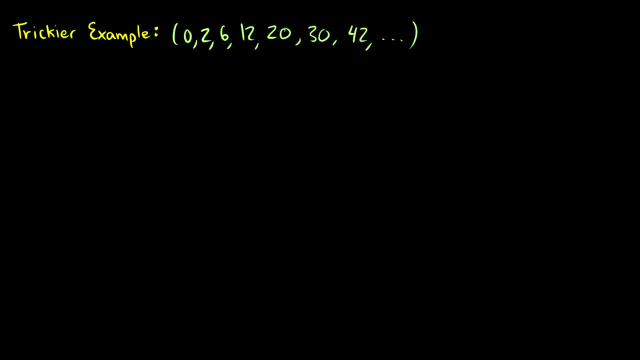 So, for instance, this sequence: 0,, 2,, 6,, 12,, 20,, 30,, 42.. I hope you can see the pattern just by looking at it. To get from the first to the second, we add 2.. 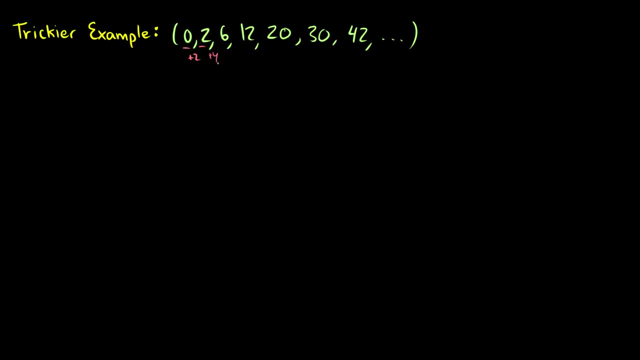 To get from the second to the third, we get plus 4, then plus 6, then plus 8, plus 12,- sorry, plus 10, so on and so forth. So another way of writing this- and I know this technique is going to seem like I'm just pulling it out of my butt- 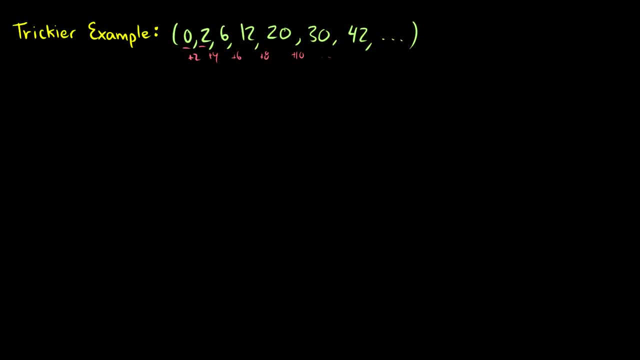 but It's hard to see, and the fact that somebody else has shown me how to do this makes it a lot easier. So would I expect you to just understand what I'm doing straight away Or how I got to this solution? No, 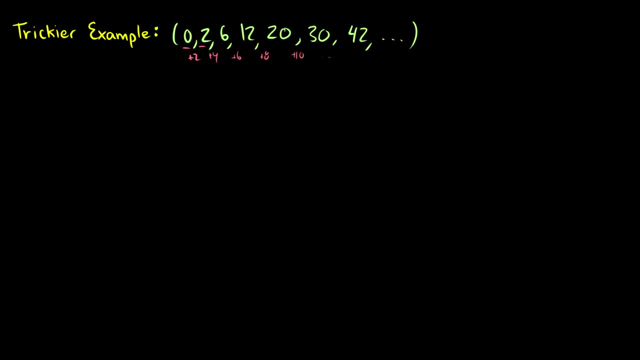 That's why you're watching a video: so you can see someone else do it and hopefully you get some insight into future questions or future examples where you see something very similar. Okay, so let's write this as a1 minus a0.. 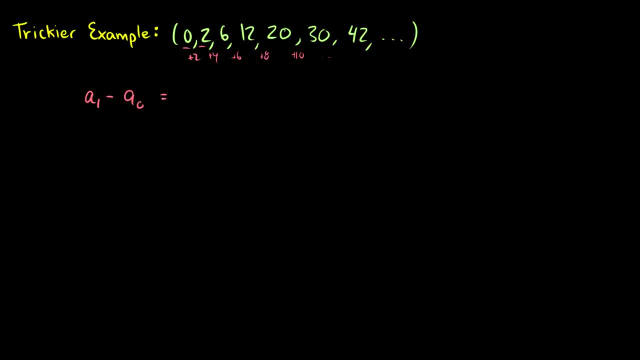 So this is 2 minus 0. This is equal to 2.. Okay, a2 minus a1 is 6 minus 2, which is 4.. Again, what I'm going to do is just to make things super clear. 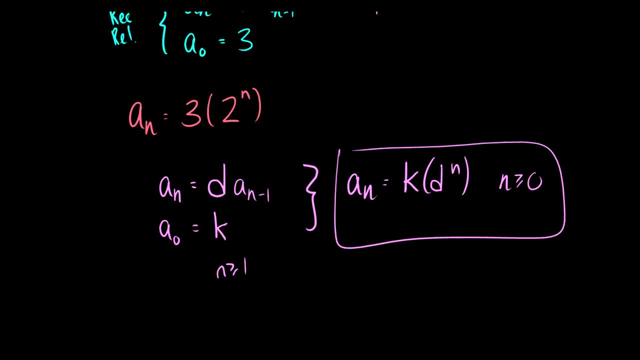 And this recurrence relation is going to be n greater or equal to 1.. So these are two different ways of looking at things. One is a recurrence relation, The other is a nice formula that allows us to compute any number without needing to know the previous numbers. 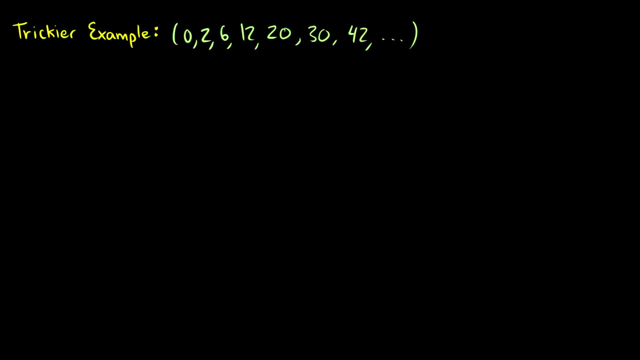 So that's great. But what can happen is we can get some more tricky examples. So for instance, this sequence: 0, 2, 6, 12, 20, 30, 42.. I hope you can see the pattern just by looking at it. 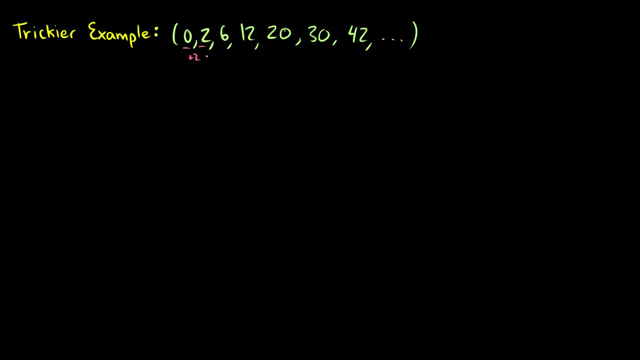 To get from the first to the second, we add 2.. To get from the second to the third, we get plus 4, then plus 6, then plus 8,, plus 12,- sorry, plus 10, so on and so forth. 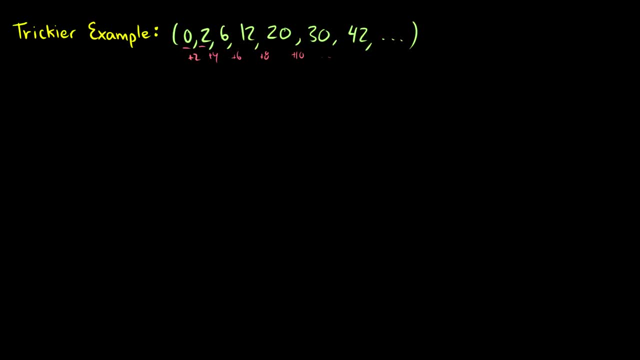 So another way of writing this- and I know this technique is going to seem like I'm just pulling it out of my butt, but It's hard to see, and the fact that somebody else has shown me how to do this makes it a lot easier- 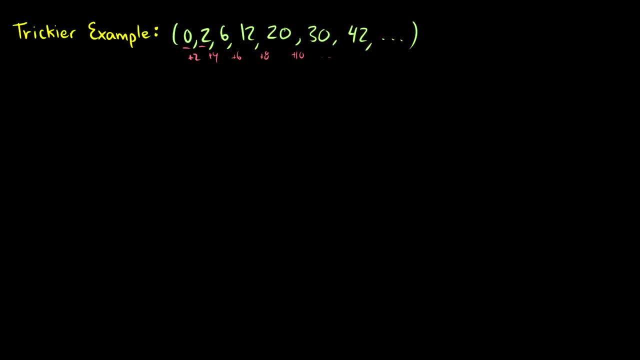 So would I expect you to just understand what I'm doing straight away Or how I got to this solution? No, That's why you're watching a video: so you can see someone else do it and hopefully you get some insight into future questions. 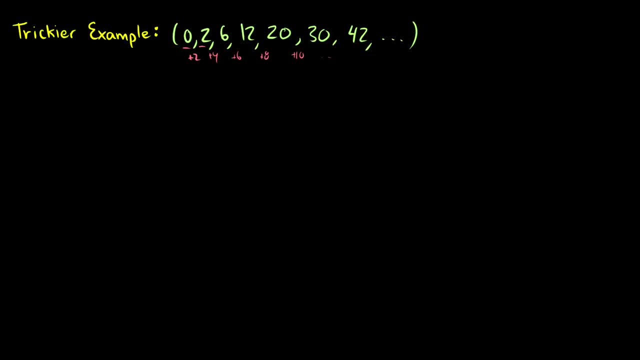 or future examples where you see something very similar. Okay, so let's write this as a1 minus a0.. So this is 2 minus 0.. This is equal to 2.. Okay, a2 minus a1 is 6 minus 2, which is 4.. 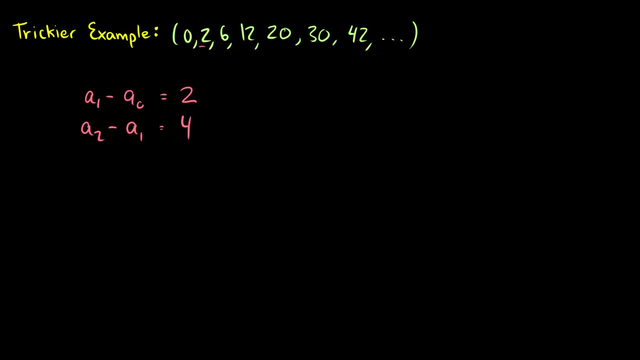 Again, what I'm going to do is just to make things super clear. I'm going to write this as a0, a1, a2, a3, a4, so on. Okay, a3 minus a2 is 12 minus 6, which is 6.. 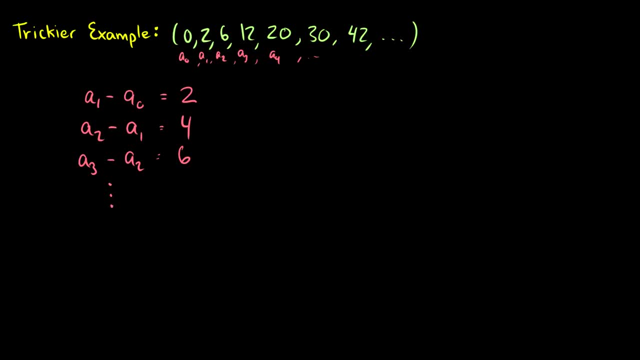 So we can see this pattern here. So, following this pattern, we can see that an minus an minus 1 is going to be 2 times n. Okay, so what we're going to do now is we're going to add all of these up. 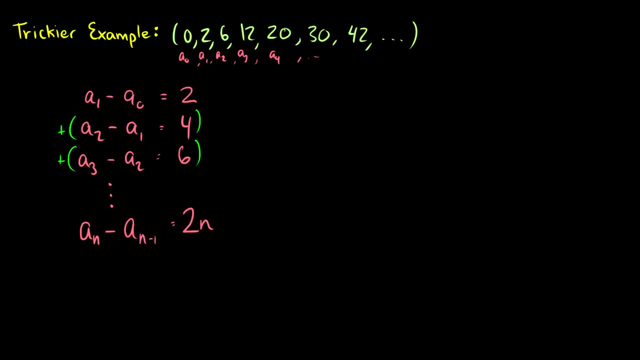 So let's add up all of these formulas and what we're going to get is, well okay, a1 minus a0.. Let's add up the left side first. So we're going to get a1 minus a0 plus a2 minus a1.. 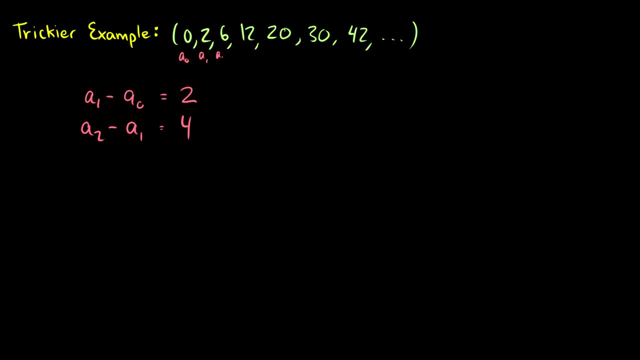 I'm going to write this as a0, a1, a2,, a3, a4, so on. Okay, a3 minus a2 is 12 minus 6, which is 6.. So we can see this pattern here. 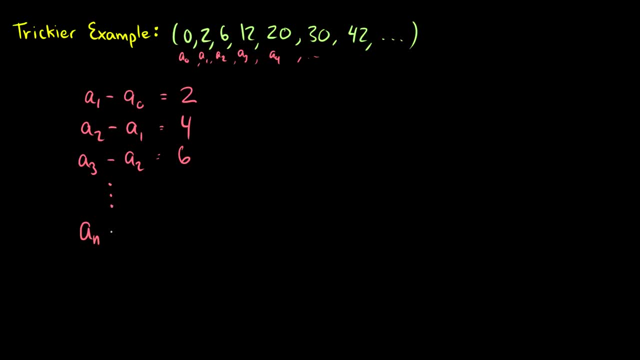 So, following this pattern, we can see that an minus an minus 1 is going to be 2 times n. Okay, so what we're going to do now is we're going to add all of these up. So let's add up all of these formulas. 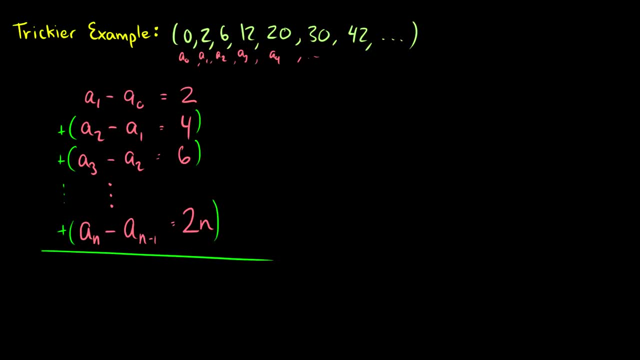 and what we're going to get is well, okay, a1 minus a0.. Let's add up the left side first. We're going to get a1 minus a0 plus a2 minus a1.. We're going to get a1 minus a1, so these a1s are going to cancel. 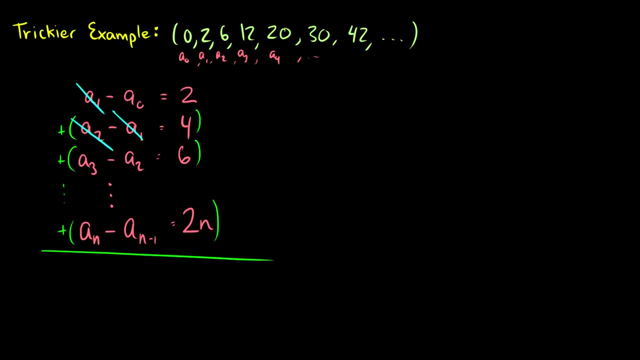 Then we're going to get a2 plus a3 minus a2.. Okay, so these a2s are going to cancel and similarly, the a3s will cancel, all the way up to the an minus 1s will cancel and we'll be left with an minus a0. 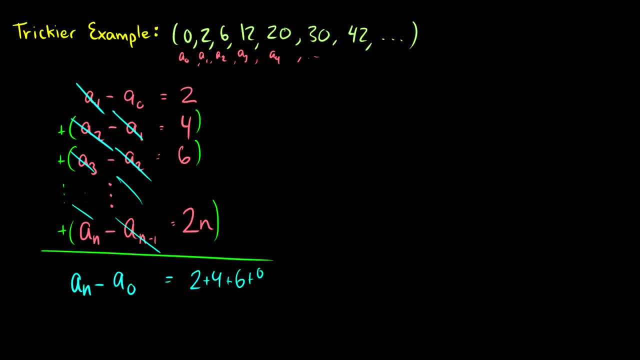 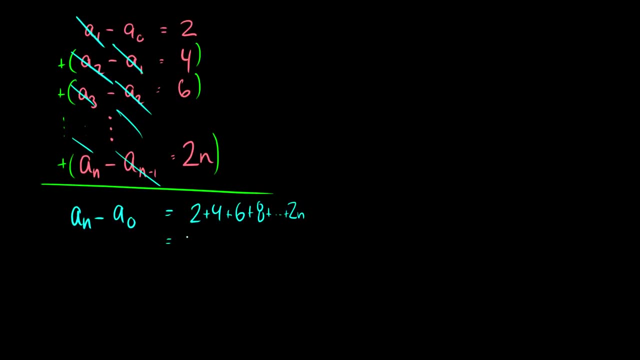 And this is going to be equal to 2 plus 4,, 6 plus 8, all the way up to plus 2n, which we can just factor out a 2.. And then we get 1 plus 2 plus all the way up to plus n. 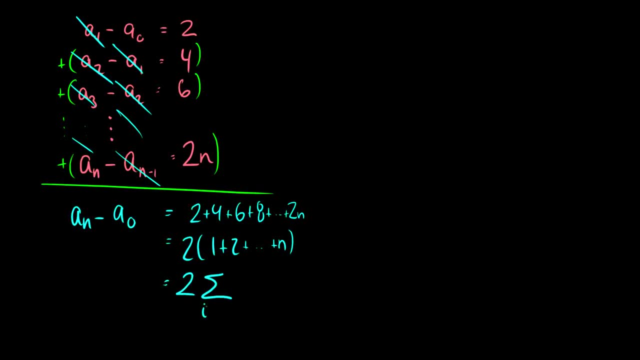 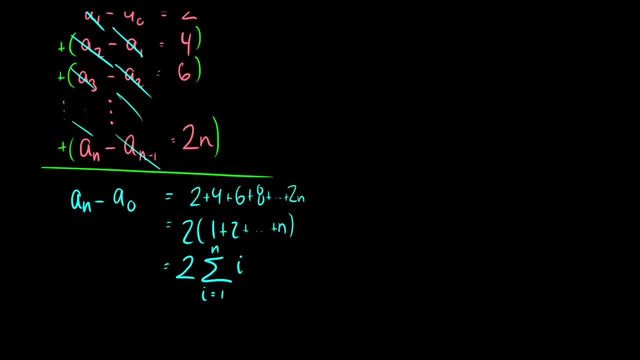 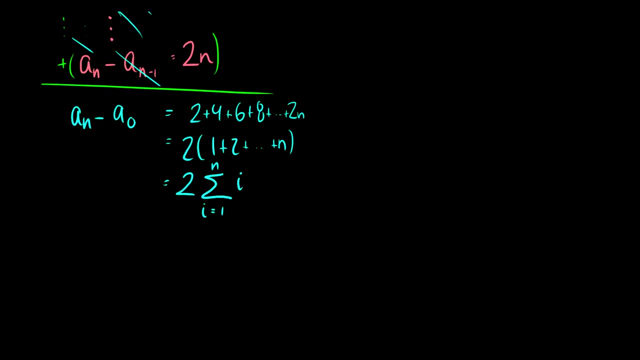 which we can write as: 2 times the sum from i goes to 1 to n of i, And if you remember this formula from a calculus course, I don't expect you to know the formula for any exam or test questions that I have on my website. 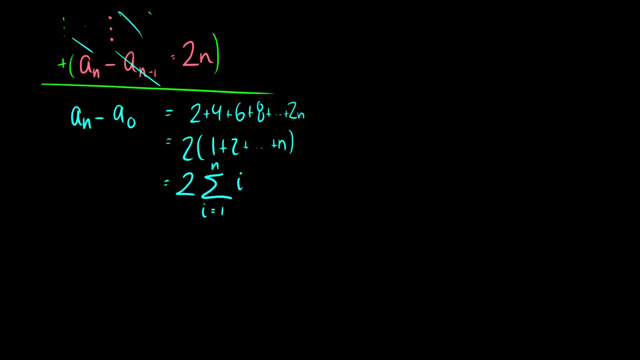 If I did, I would give you the formula. So whether you need to know this formula or not depends on your professor. But this is the same thing as 2 times n times n plus 1 over 2.. So this simplifies to n times n plus 1.. 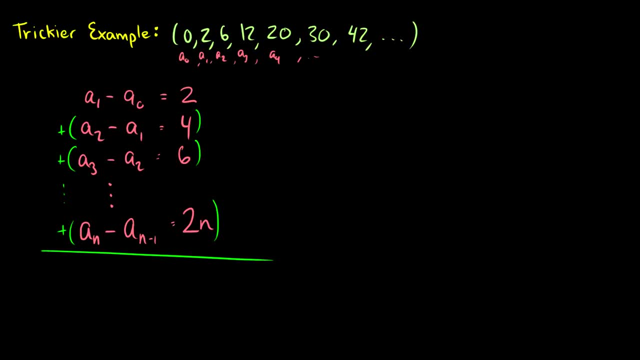 We're going to get a1 minus a1.. So these a1s are going to cancel. Then we're going to get a2 plus a3 minus a2.. Okay, so these a2s are going to cancel And similarly, the a3s will cancel all the way up for the an minus 1s will cancel. 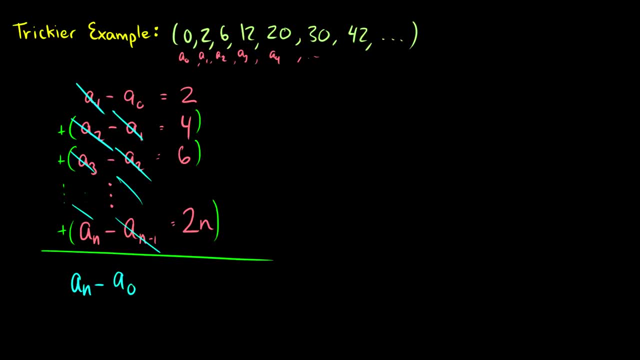 and we'll be left with an minus a0.. And this is going to be equal to 2 plus 4 plus 6 plus a1 minus a0.. Okay, so this is going to be equal to 2 plus 4 plus 6 plus a1 minus a0. 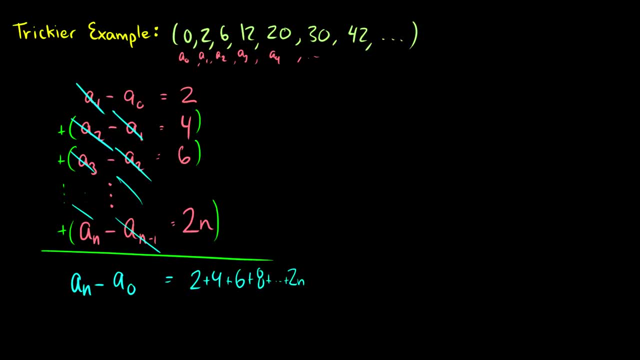 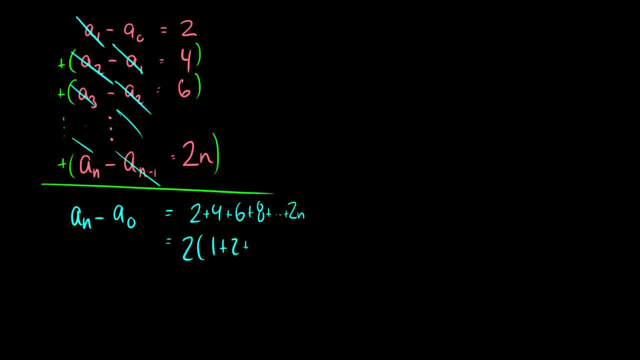 Okay, so this is going to be equal to 2 plus 4 plus 6 plus 8, all the way up to plus 2n, which we can just factor out a 2, and then we get 1 plus 2 plus all the way up to plus n. 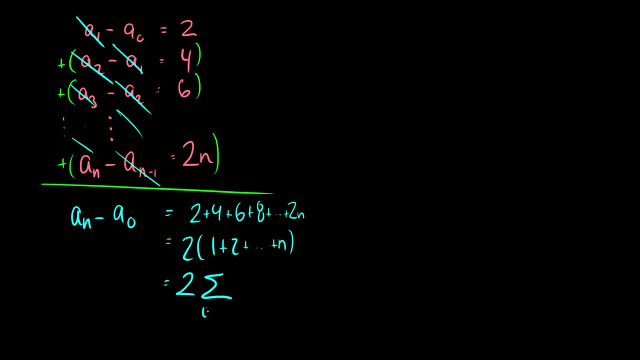 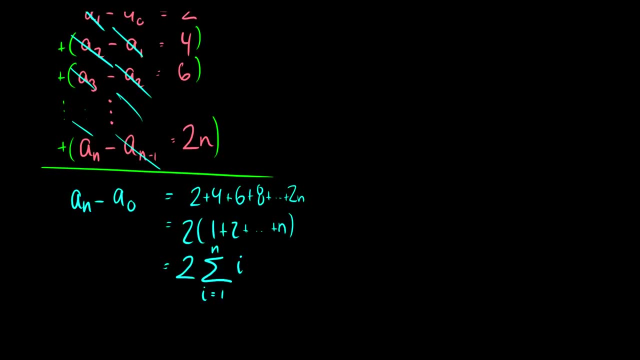 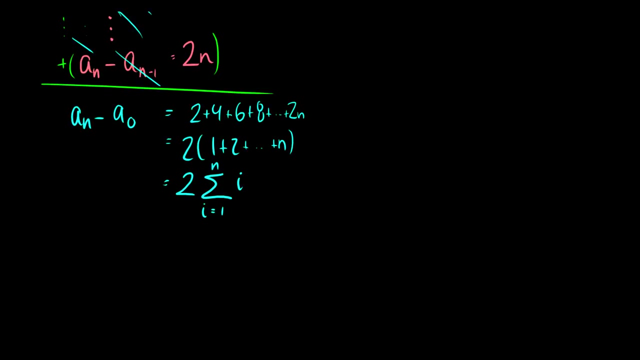 which we can write as: 2 times the sum from i goes to 1 to n of i, And if you remember this formula from a calculus course, I don't expect you to know the formula for any exam or test questions that I have on my website. 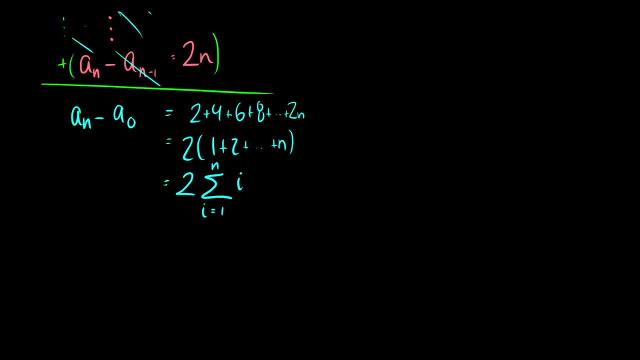 If I did, I would give you the formula. So whether you need to know this formula or not depends on your professor. But this is the same thing as 2 times n times n plus 1 over 2.. So this simplifies to n times n plus 1.. 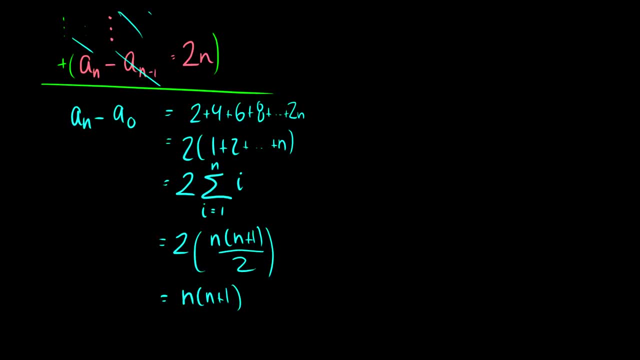 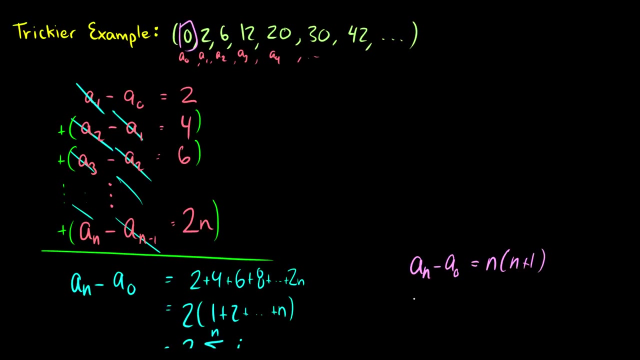 So the recurrence relation solution is an: a1 minus a0 is equal to n times n plus 1.. What is a0?? Okay, let's take a look here. A0,, oh, 0,. okay, So an is equal to n times n plus 1.. 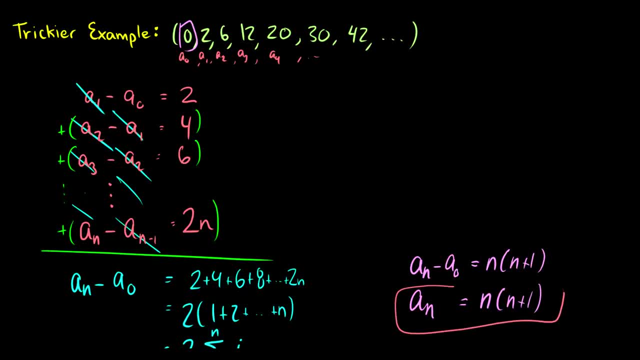 So this is the solution. So that might have been a little bit fast, and it's going to be fast because, well, this is a unique way of looking at recurrence relations that you probably haven't seen before: adding up a bunch of equations and summarizing. 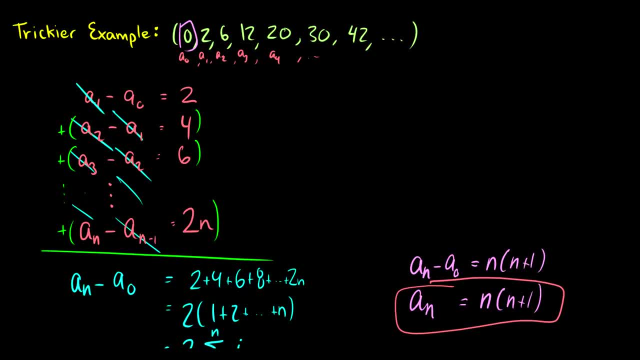 So instead- well, first we should check to make sure it works- Let's pick a6.. So a6, we know, is equal to 42. That's this number here. So a6 is going to be 6 times 6 plus 1,. 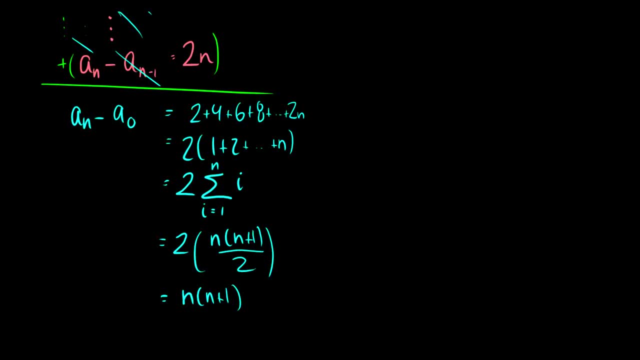 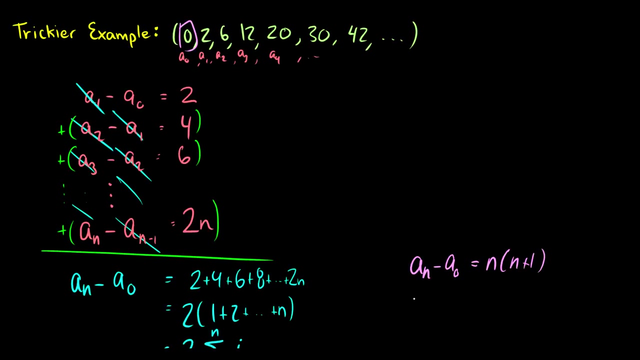 So The recurrence relation solution is: an minus a0 is equal to n times n plus 1.. What is a0?? Let's take a look here: a0. Zero, OK. So an is equal to n times n plus 1.. 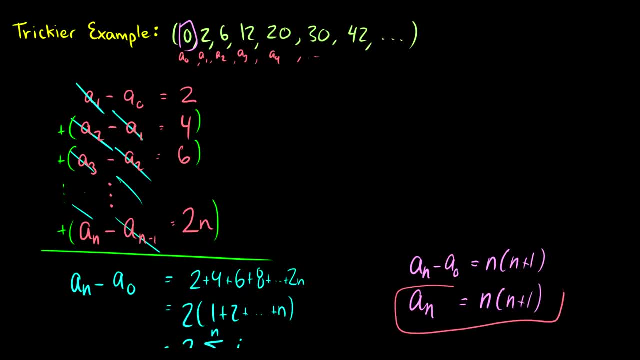 So this is the solution. So that might have been a little bit fast, And it's going to be fast Because, Well, This is a unique way of looking at recurrence relations that you probably haven't seen before: adding up a bunch of equations and summarizing. 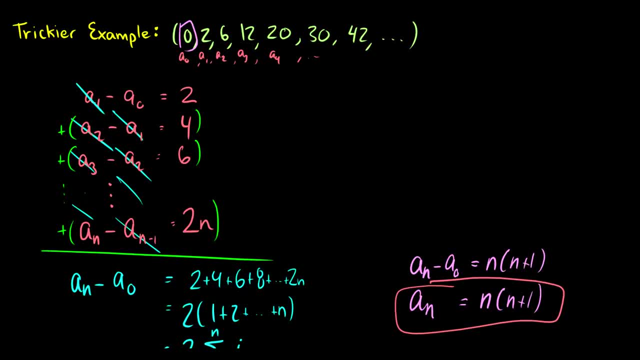 So instead- well, first we should check to make sure it works. Let's pick a six. So a six, we know, is equal to 42. That's this number here. So a six is going to be six times six plus one. 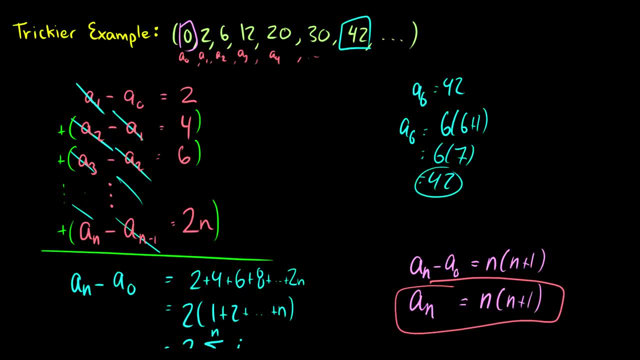 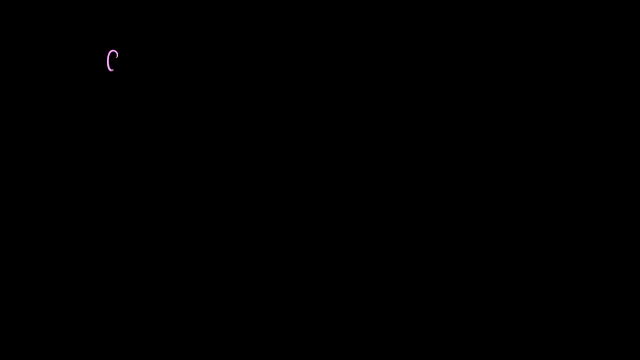 which is six times seven, which is 42. So it works Very cool. Okay, here's a nice way of looking at things. When we have any any recurrence relation, that looks like an minus. an minus one is equal to some number, okay. 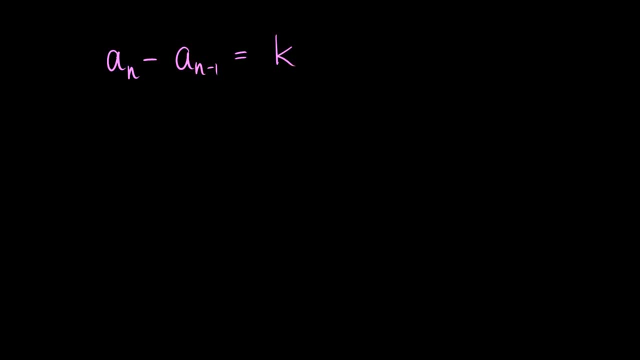 What we can do is say that, well, we should probably define a zero to be some number c, and this is for n, greater or equal to one. If we ever have any relation of this form, this is okay. there we go. 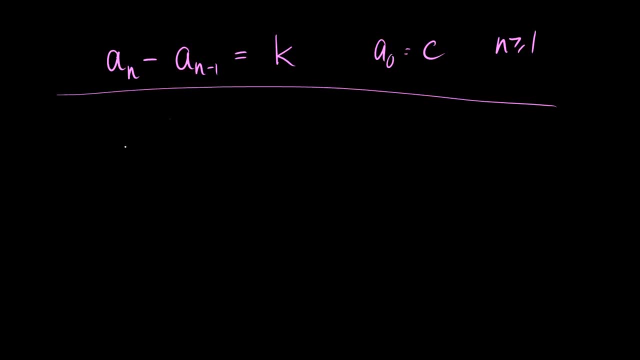 This is equal to. so an is going to be equal to a zero plus the sum, as i goes from one to n, of k. So in our previous example we had an minus. well, let's do this in a different color. We have an minus. an minus one is equal to two times n. 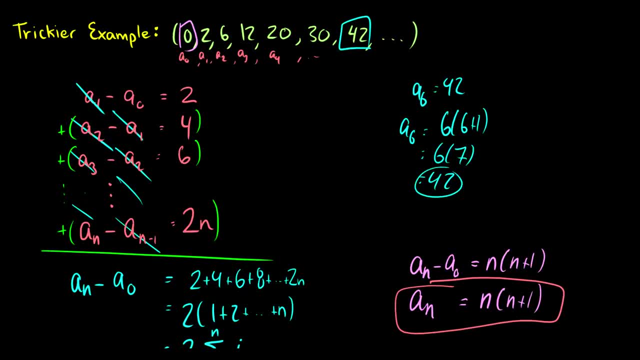 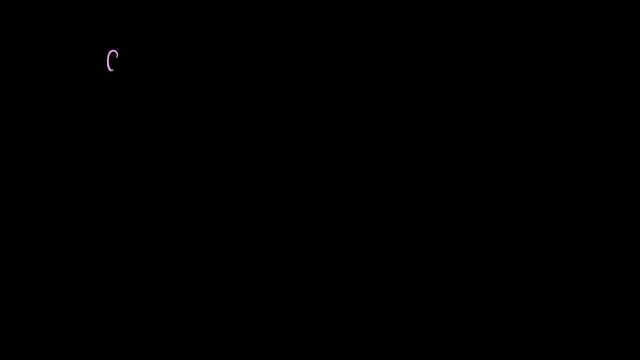 which is 6 times 7, which is 42. So it works Very cool. Okay, here's a nice way of looking at things. When we have any any recurrence relation, that looks like an minus an minus 1 is equal to some number, okay. 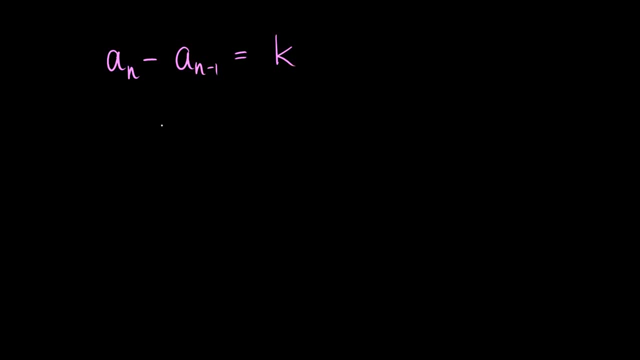 what we can do is say that, well, we should probably define a0 to be some number c, and this is for n greater or equal to 1. If we ever have any relation of this form, this is okay. there we go. 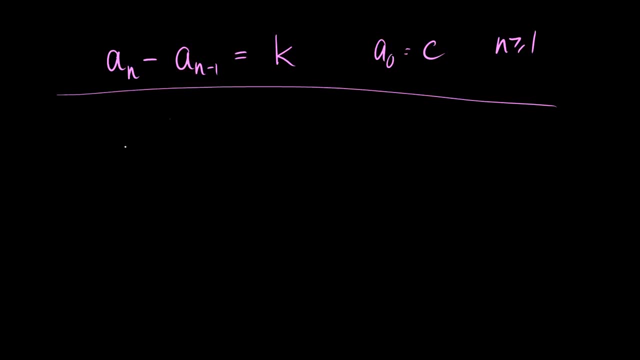 This is equal to. so an is going to be equal to a0, plus the sum as i goes from 1 to n, plus the sum as i goes from 1 to n and plus the sum of k. So in our previous example, 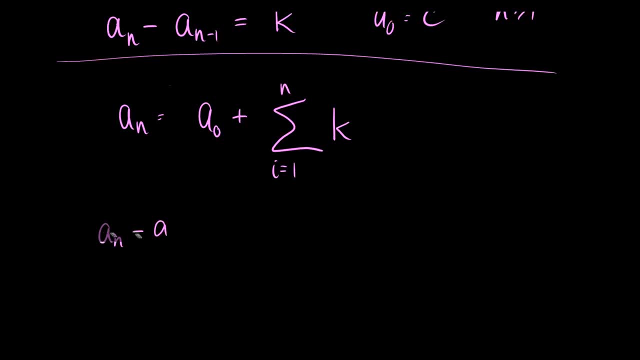 we had an minus. well, let's do this in a different color. We have an minus. an minus 1 is equal to 2 times n We had. a0 is equal to 0, for n greater or equal to 1.. This an is equal to. 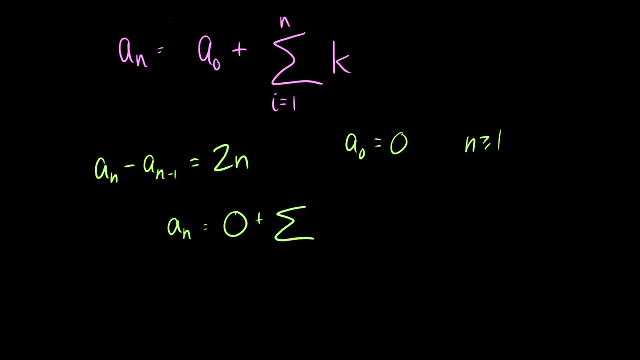 0,, which is 0, plus the sum, as i goes from 1 to n, of 2 to the n. We can simplify this and say this is 2 times the sum of i equals 1 to n of n. we just factor out the 2,, and this is equal to 2. 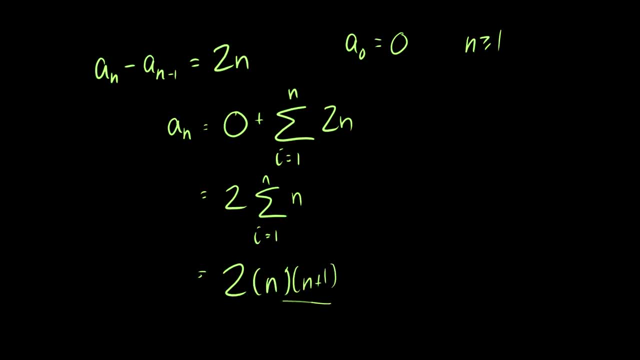 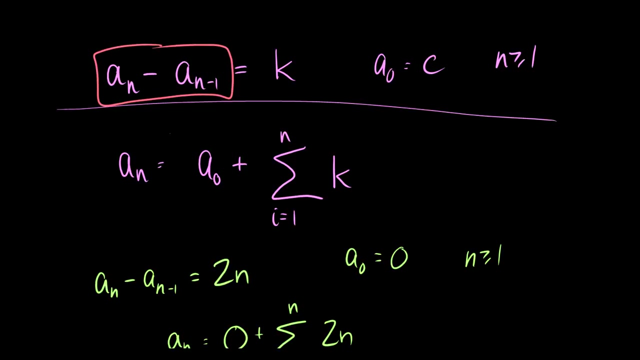 times n times n plus 1, all over 2, which we know cancels and we get n times n plus 1.. So this is another little formula for recurrence relations that is pretty important. This- sorry, this should be a little bit higher. This requires a n minus a n minus 1.. If you have a number here like 3,, 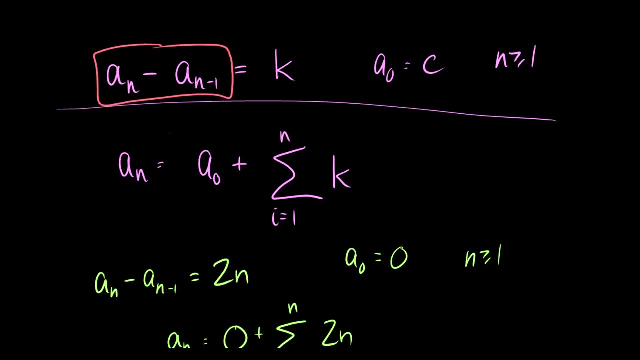 it does not work. We will cover that next time, but for now there's your solution. That might have been tricky, so I definitely suggest going over this very slowly. In fact, for those of you who are still saying where the hell did that, 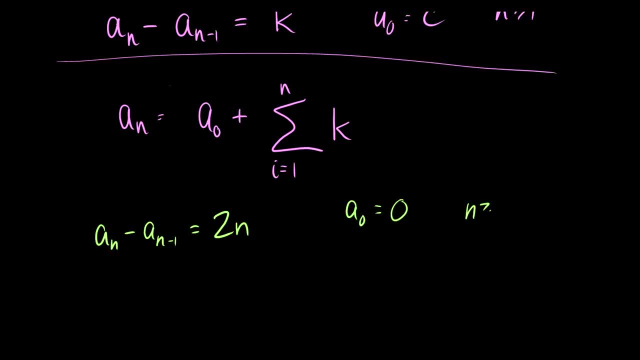 We had, a zero is equal to zero. This is a minus of two. Let's do it one more time for n greater or equal to one. This an is equal to a zero, which is zero plus the sum, as i goes from one to n, of two to the n. 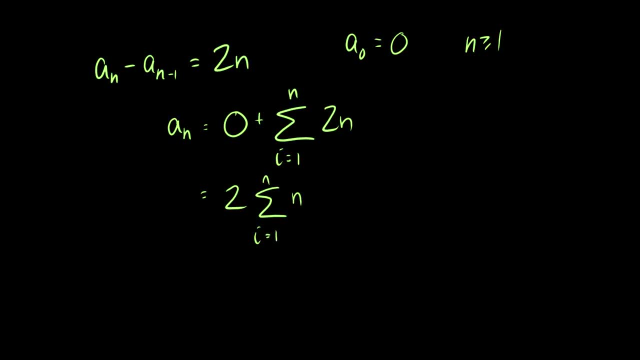 We can simplify this and say this is two times the sum of i equals one to n of n. We just factor out the two and this is equal to two times n times n plus one, all over two, which we factor out. 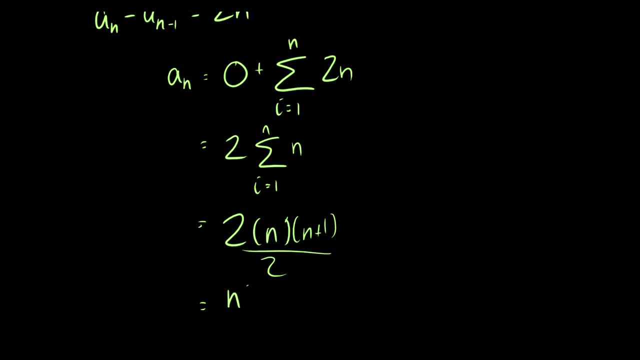 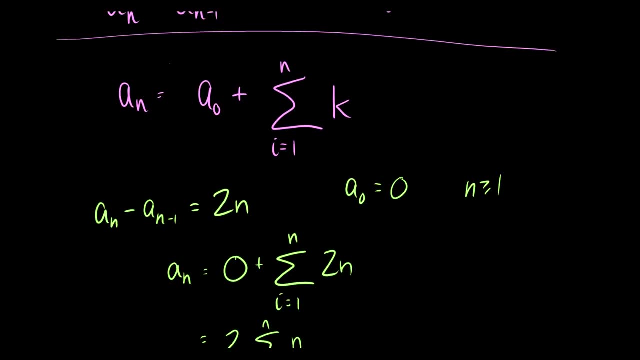 So this is equal to something else right, which we know cancels, and we get n times n plus 1.. So this is another little formula for recurrence relations that is pretty important. This- sorry, this- should be a little bit higher. This requires: 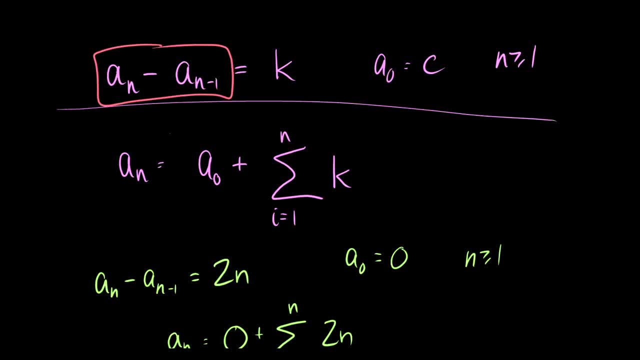 an minus, an minus 1.. If you have a number here like 3, it does not work. We will cover that next time, but for now, there's your solution. That might have been tricky, so I definitely suggest going over this very slowly. In fact, for those of you who are still saying: where the hell? 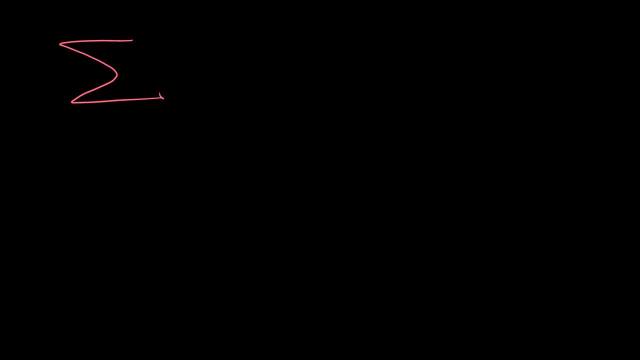 did that sum proof come from Oh? e of i equals 1 to n. of i is equal to n times n plus 1 over 2.. You should know this. Why does this work? Okay, here's a proof of why this works. Let's do. 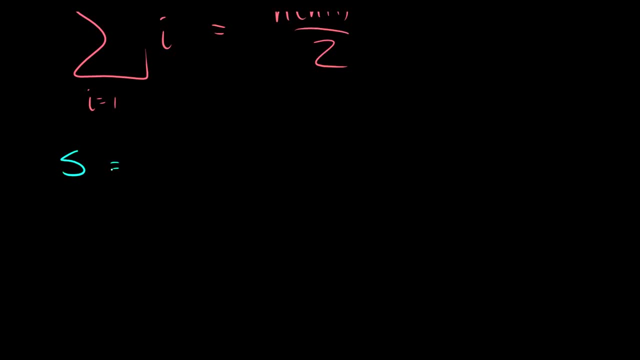 this, This impromptu proof We're going to take s. This is going to be equal to 1 plus 2 plus 3 plus 4, all the way up to n. We're going to take the same sequence, except we're going to take it backwards. 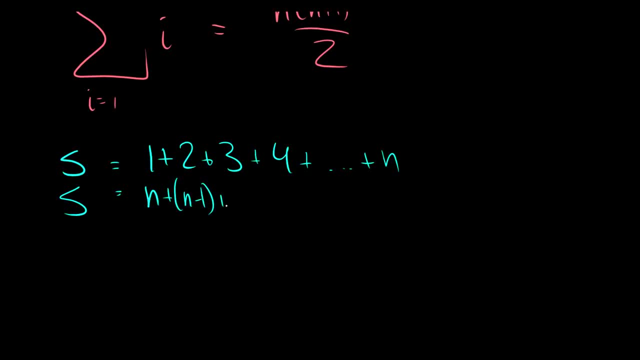 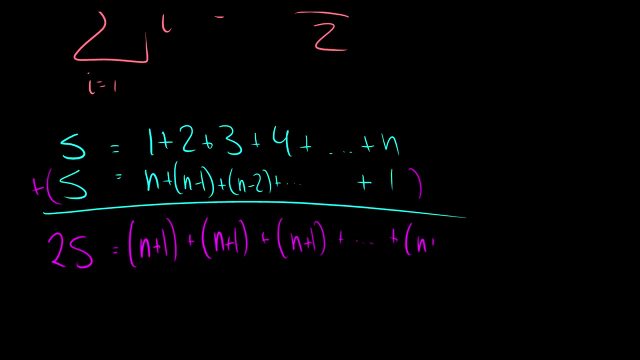 So this is n plus n minus 1 plus n minus 2, all the way up to plus 1.. Okay, let's add these together. Let's add this whole sequence together. So 2s is equal to okay. well, 1 plus n is n plus 1.. n minus 1 plus 2 is n plus 1.. n minus 2 plus 3 is going to be n plus 1.. So this is going to add up to the last number here, which is n plus 1, which is n plus 1.. Again, I'm just adding vertically here. 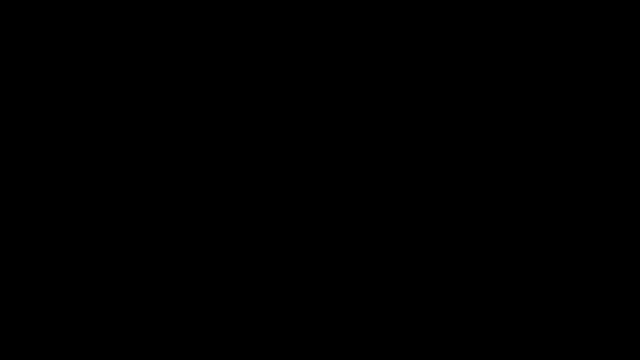 sum come from: E of i equals 1 to n of i is equal to n times n plus 1 over 2.. You should know this. Why does this work? Okay, here's a proof of why this works. Let's do this. impromptu proof We're going to take. 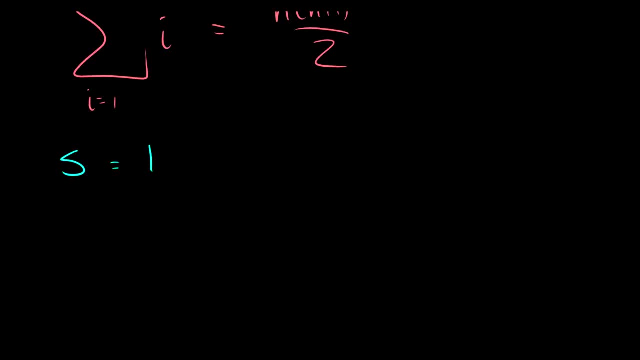 s. This is going to be equal to 1 plus 2 plus 3 plus 4, all the way up to n. We're going to take this same sequence, except we're going to take it backwards. So this is n plus n minus 1 plus n minus 2. 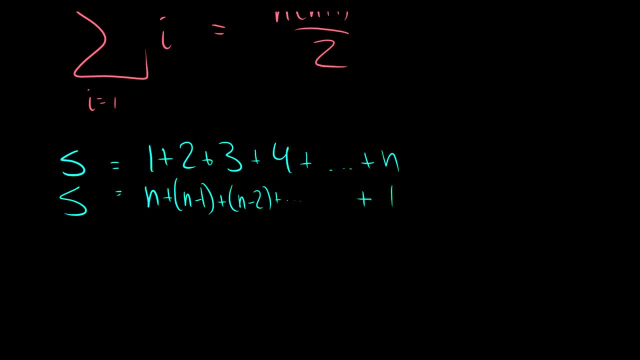 all the way up to plus 1.. Okay, let's add these together. Let's add this whole sequence together. So 2s is equal to. okay. well, 1 plus n is n plus 1.. n minus 1 plus 2 is n plus 1.. 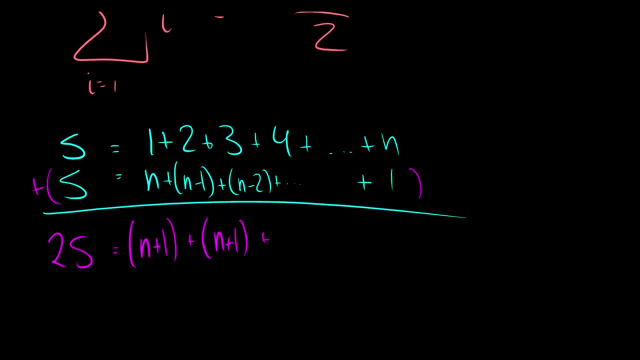 n minus 2 plus 3 is going to be n plus 1, so this is going to add up to the last number here, which is n plus 1, which is n plus 1 again. I'm just adding vertically here, okay, so how many numbers? 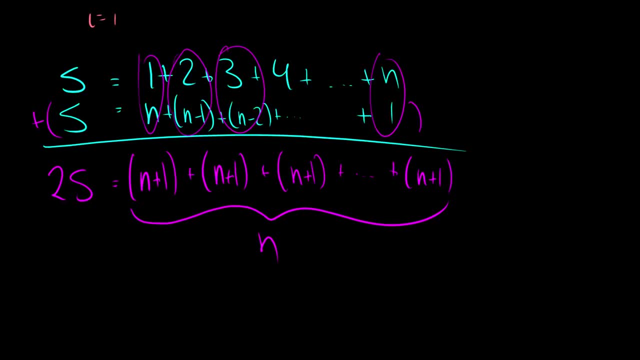 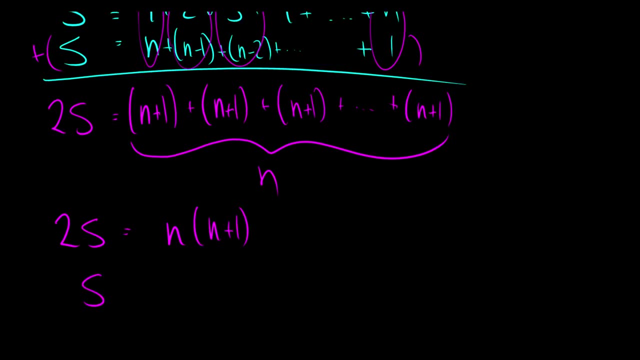 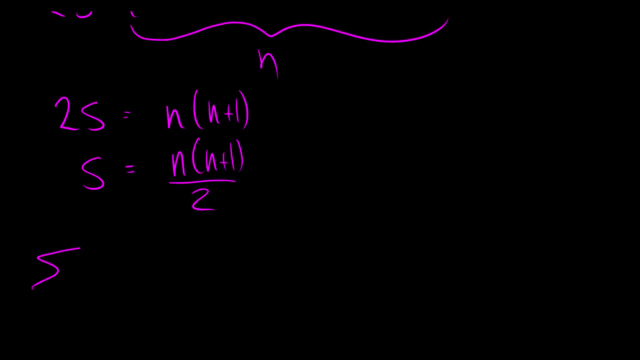 are there? well, there are n numbers, so this is added n times. so, really, 2s is equal to n times n plus 1, so that means that s is equal to n times n plus 1 over 2, so this is equal to the sum of i. 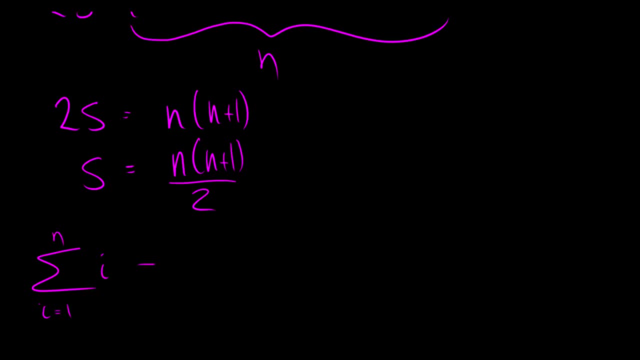 equals 1 to n of i, and that's n times n plus 1 over 2. there you go. that is the proof of the sum. for those of you wondering where that came from, if you ever needed this, I would provide it. your prof might not. so that was the proof of the sum for this lesson. 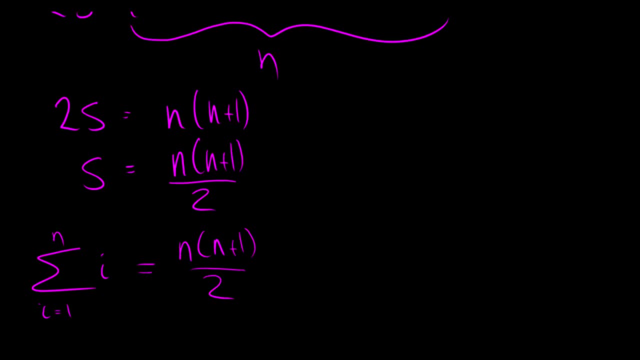 So that was the proof of the sum for this lesson. So that was some very simple recurrence relations. I say simple not because they should be easy to you, because they shouldn't be if you're just seeing this for the first time, but simple because the next videos are going to be much, much harder. so if you have any questions, leave them in the